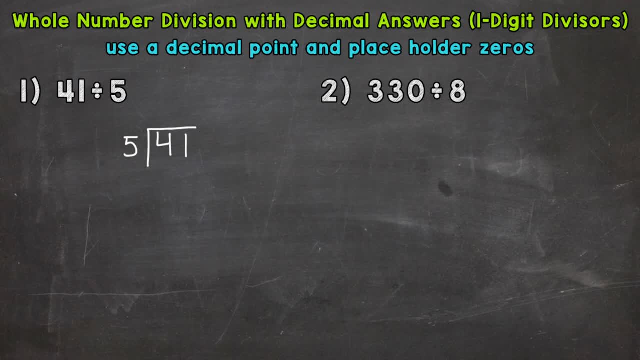 problem. So we start with divide. So 4 divided by 5. How many whole groups of 5 can we pull out of 4?? Well, we can't. So we need to look at the 41. So we have 41 divided by 5. And we're going to 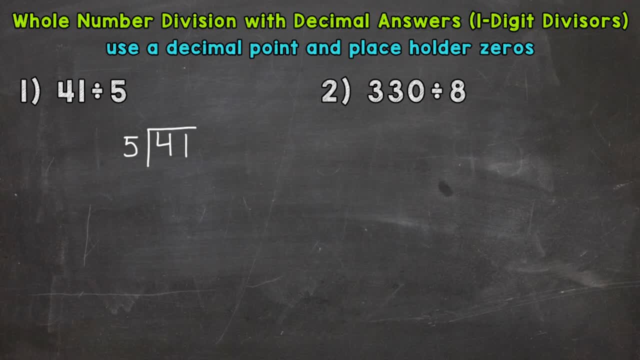 5. How many whole groups of 5 out of 41? 8. That gets us to 40. Now we multiply 8 times 5? 40. Subtract, We get 1.. So 8 remainder 1 would be the correct answer, but we want this in decimal form. 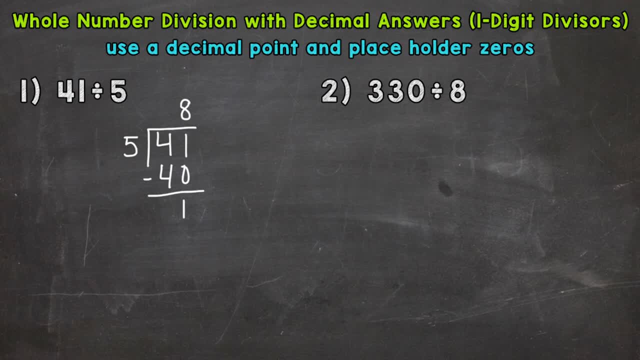 So what we're going to do, we're going to use a decimal point, place it after the 41, and then bring that straight up into your answer, And we're going to use a placeholder 0 to the right of that decimal point. That way we have. 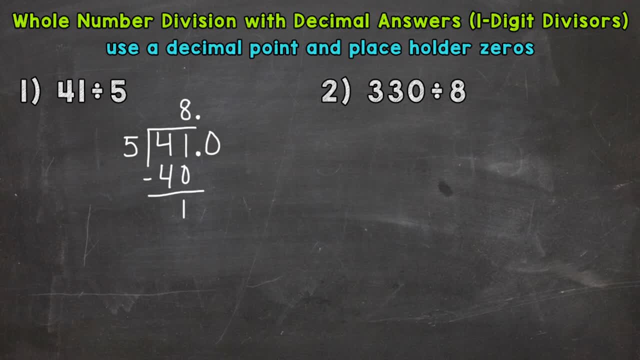 something to bring down and continue our division process. Placing a 0 to the right of a decimal point does not change the value of the problem, So that 0, we still have 41 there, So it's okay to use that placeholder 0. Let's bring that down and continue. So now we have 10 divided by 5.. 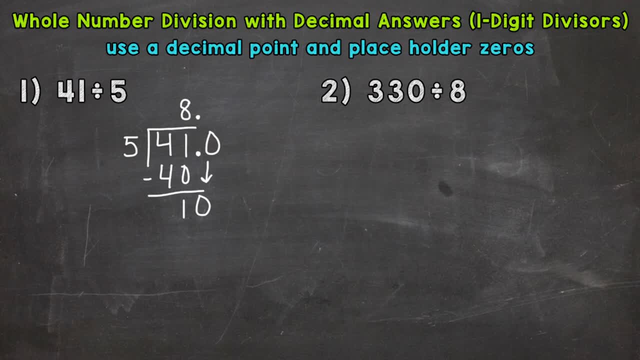 So how many whole groups of 5 out of 10? 2. Let me extend that there. Now we multiply 2 times 5 is 10.. Subtract And we get that clean, cut 0.. That's what we're looking for Once we get that. 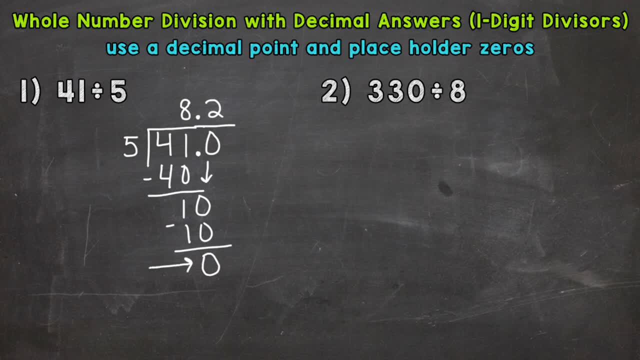 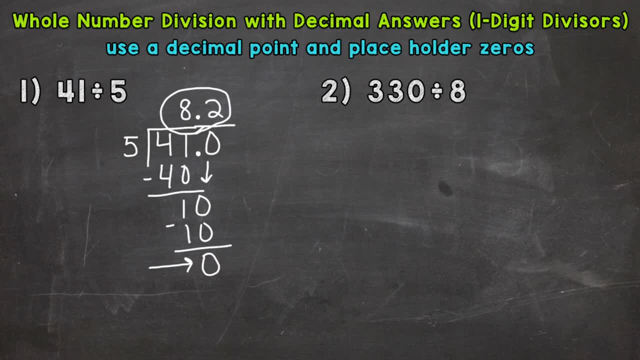 We have 330 divided by 8.. So let's set that up: 330 divided by 8.. Let's start with divide. So 3 divided by 8. How many whole groups of 8 out of 3?? We can't do that, So we need to use the 33.. 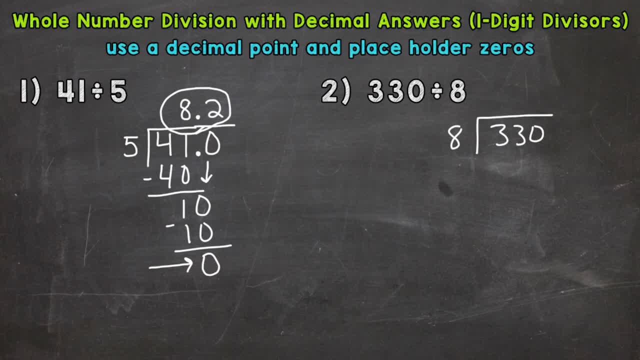 How many whole groups of 8 out of 33? 4. That gets us to 32.. 4 times 8, 32.. Subtract We get 1 and bring down our 0. So how many whole groups of 8 out of 10? 1.. 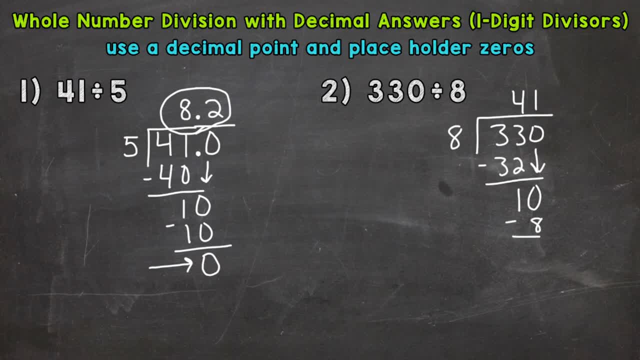 1 times 8 is 8. Subtract And we get 2.. So 41 remainder 2 is our answer. But again, we want decimal form. So what we do? we place a decimal after the whole number. bring that straight. 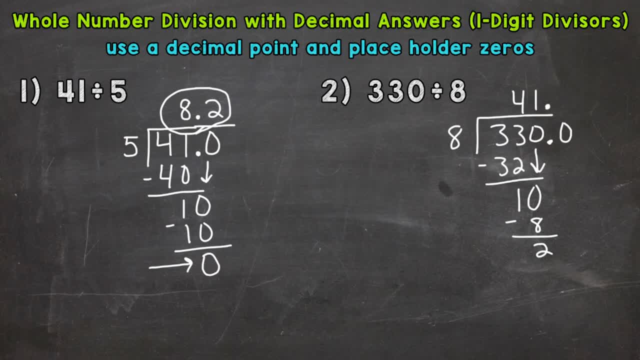 up into our answer And we use placeholder zeros to continue the process until we get a clean cut 0.. Bring this 0 down so we can continue. So we have 20 divided by 8.. How many whole groups of 8 out of 20? 2. I'll extend this again. So 2 times 8 is 16.. Subtract, We get 4.. So we did not get a 0. 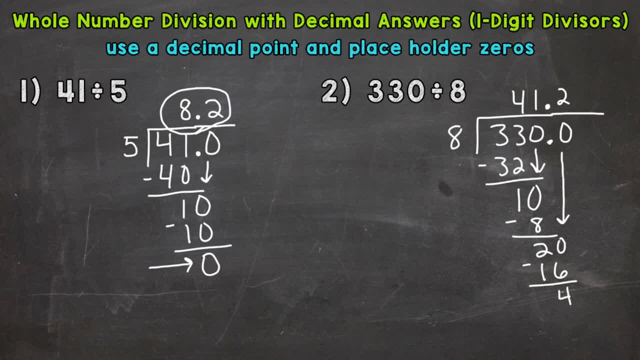 So we need to continue with Placeholder zeros until we get to that 0. So let's put another 0. This still isn't changing the value of the problem. So we are now able to bring this 0 down and continue our process. 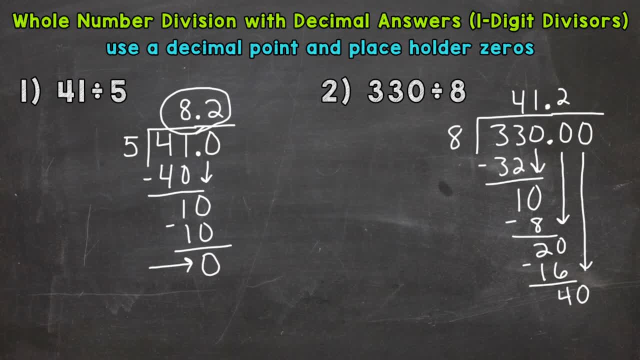 So we have 40 divided by 8. How many whole 8s out of 40?? Well, 5.. And that hits 40 exactly. So 5 times 8, 40. Subtract And we get that 0. And that lets us know that we are. 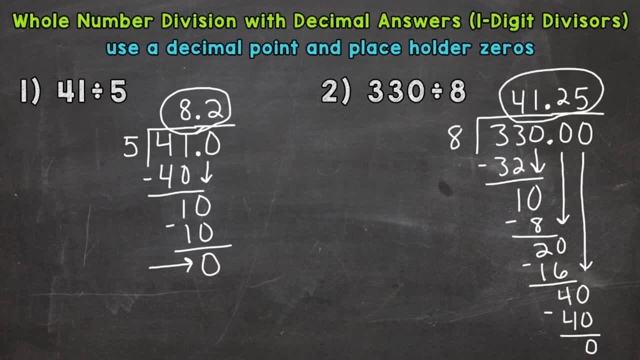 done So our answer is 41 and 25 hundredths. So there you have it. There's whole number division with decimal answers. Use decimal points and placeholder zeros to continue through the process until you get that clean, cut 0.. I hope that helped. Thanks so much for watching. Until next time, peace.